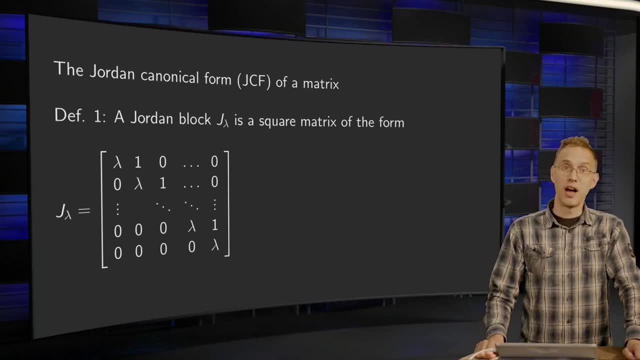 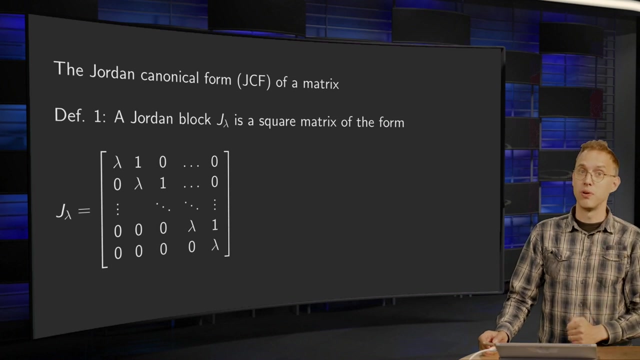 In this video we will take a look how such a matrix in Jordan canonical form looks like, And we will see that any matrix is in fact similar to such a Jordan canonical form. So let us take a look. So in order to define a Jordan canonical form of a matrix, say GCF, we first have to define a so-called Jordan block. 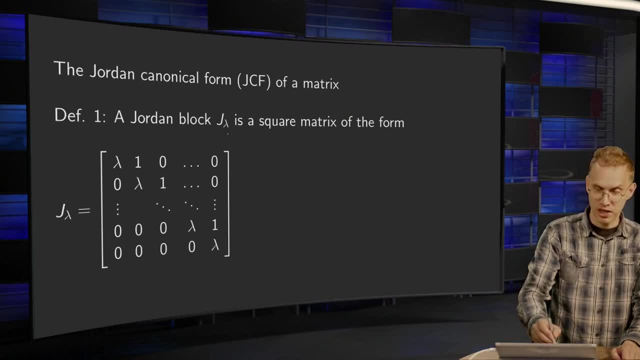 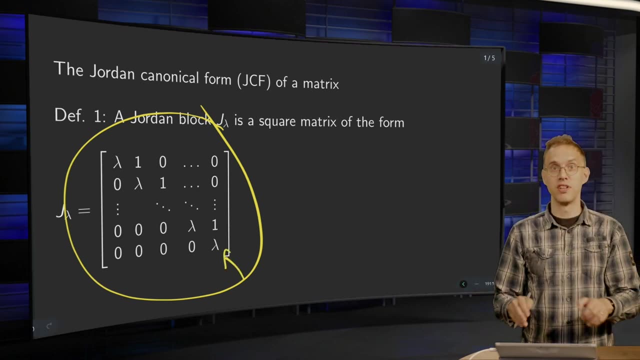 So a Jordan block is a square matrix like this. It has lambda's on the diagonal and then ones above it, So it is quite close to a diagonal matrix. The lambda's are on the diagonal all the same, Only the ones are above, and apart from that we have zeros. 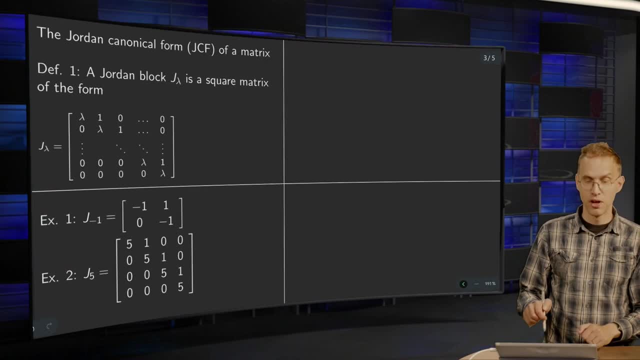 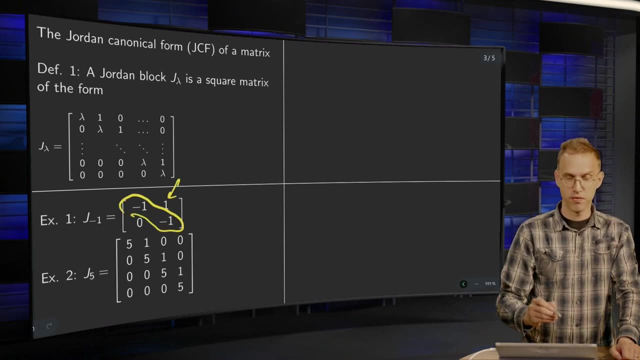 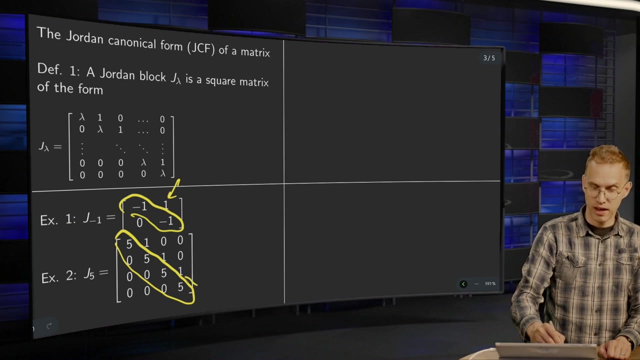 So let us take a look at a few examples. For example, a 2x2 Jordan block- Here we have the minus ones on the diagonal and the one above. And a 4x4 Jordan block, for example. Here we put fives on the diagonal and the ones above. 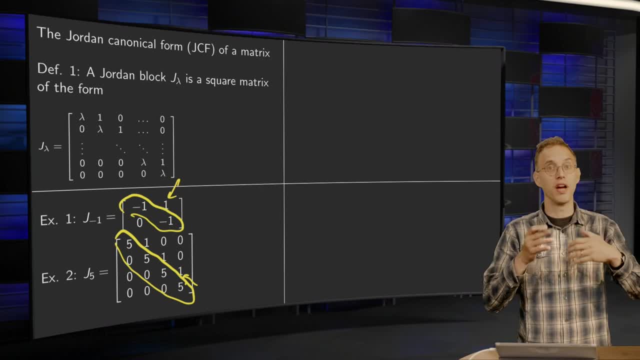 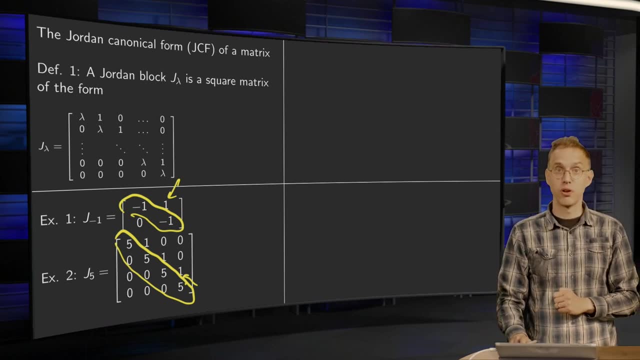 So you can really recognize easily whether we have a Jordan block or not. Now we know what a Jordan block is And then we can define what the Jordan canonical form of a matrix is, That is, a matrix which just contains a number of Jordan blocks. 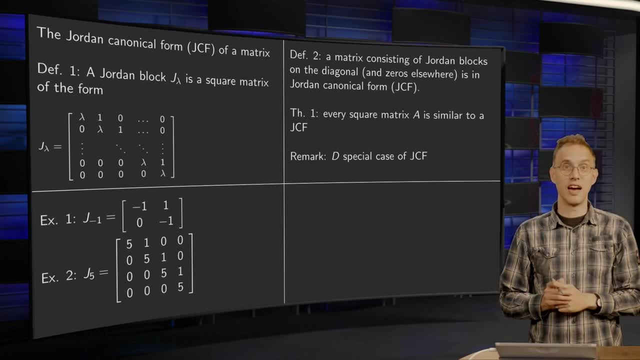 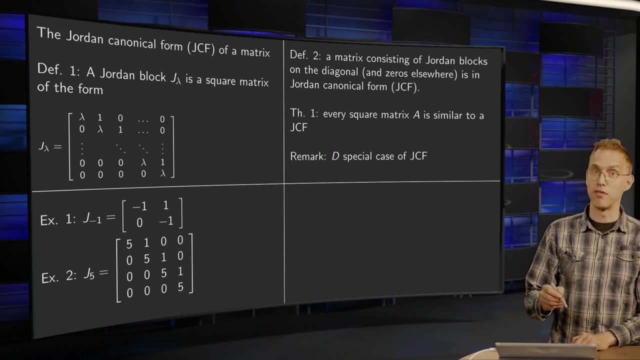 So Jordan block, Jordan block, Jordan block. That is the idea. Jordan blocks on the diagonal and apart from that, everywhere zeros. So the Jordan canonical form of a matrix contains all blocks of these forms. So that is the idea. 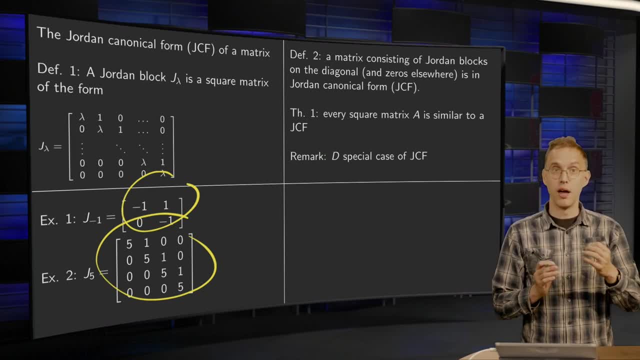 And then theorem 1, which is a principle. A pretty difficult proof, by the way, is that every square matrix is in fact similar to a Jordan canonical form. So small remark: A special case of a Jordan canonical form is if you have only 1x1 Jordan blocks. 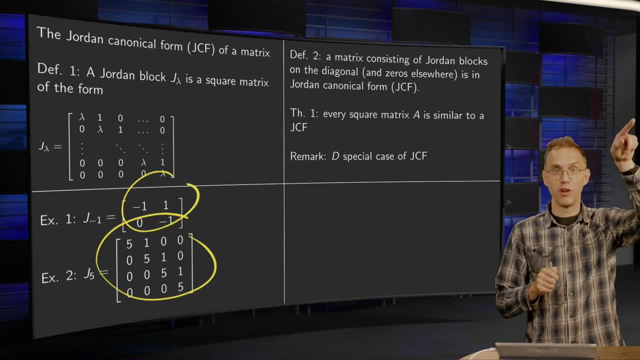 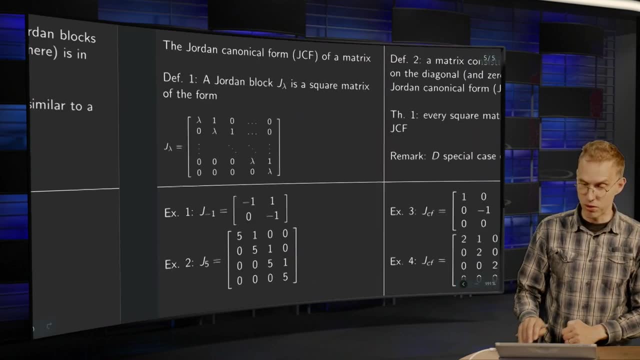 So if you have only 1x1 Jordan blocks, there are no ones above, So you have only numbers on the diagonal. So diagonalization is a special case of the Jordan canonical form. So let us take a look at a few examples. 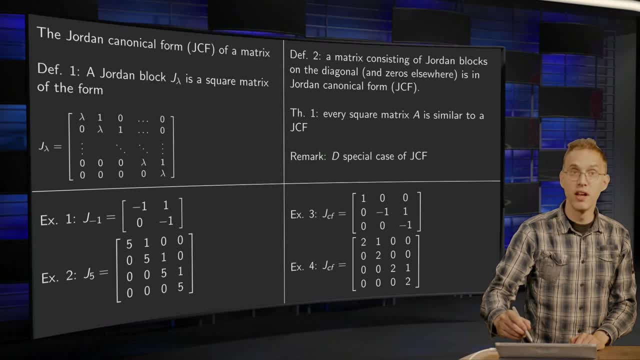 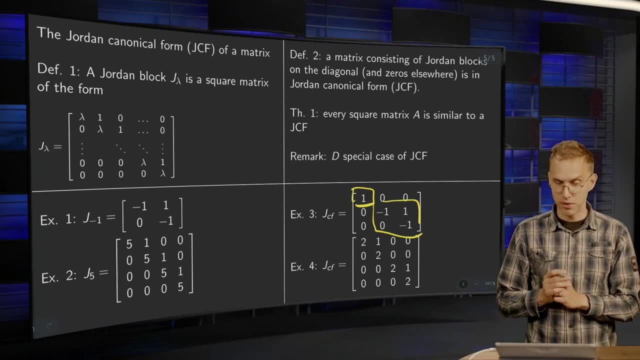 Here we have a Jordan canonical form with 2 Jordan blocks: Here the first 1x1 block And here the second 2x2 block. So that is an example of a Jordan canonical form. And here we have another example.